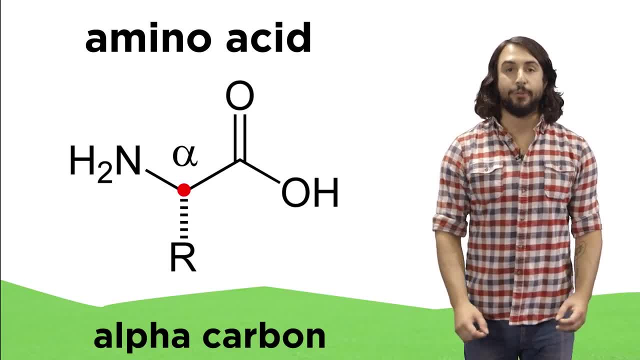 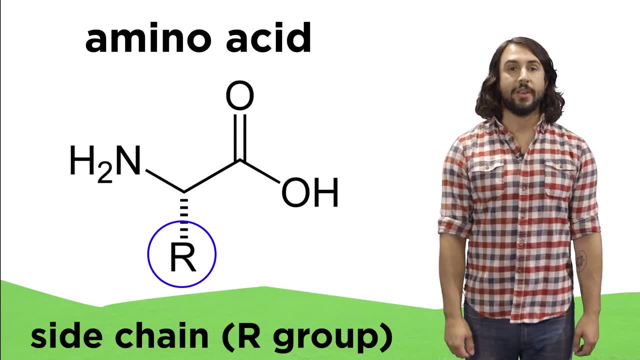 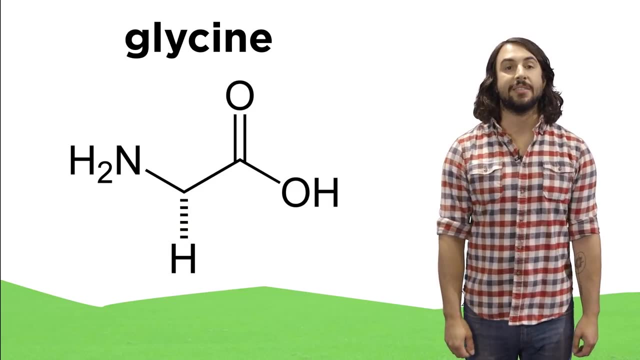 The carbon in between those functional groups, which we call the alpha carbon, will bear a side chain, sometimes referred to as an R group. This is a group that varies depending on which amino acid we are looking at. If the R group is just a hydrogen atom, we call this amino acid glycine. 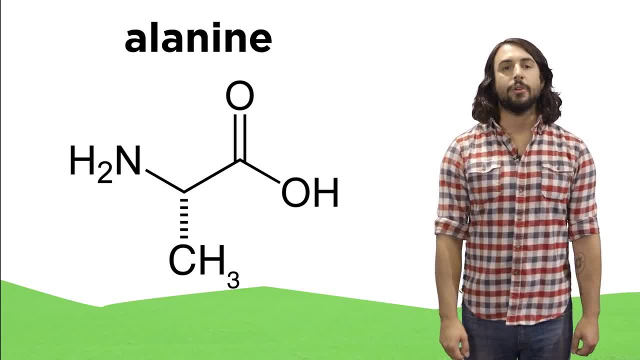 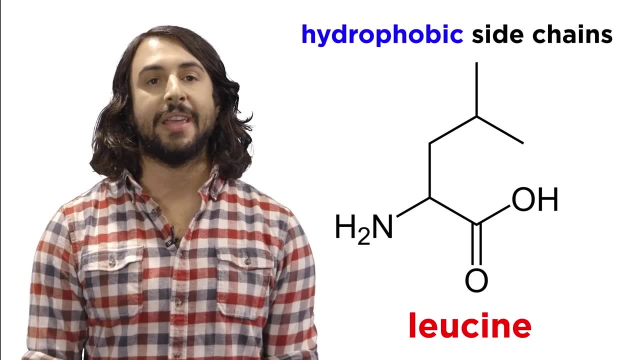 If it's a methyl group, we call this allylate. There are about 20 of them and they have a wide variety of R groups that can be put into different categories. Some of them will be hydrophobic, like leucine. 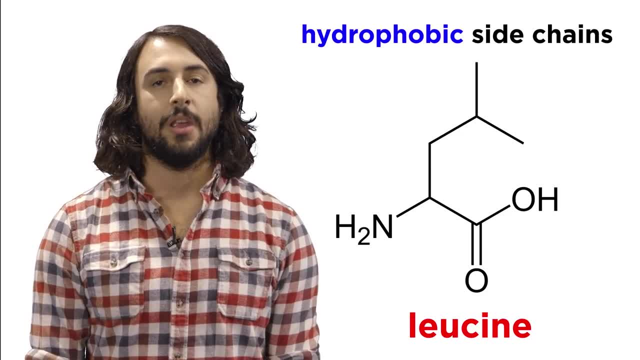 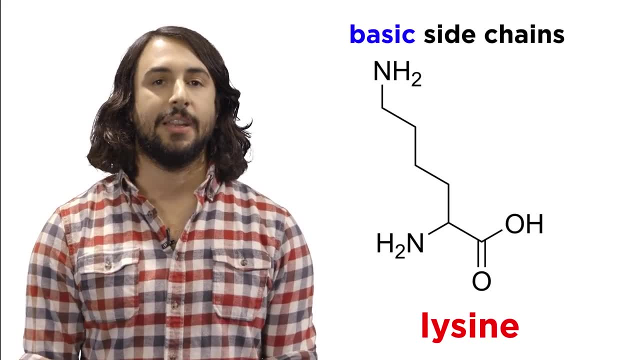 These are the ones with R groups that are alkyl substituents. Some of them have R groups that are aromatic, like phenylalanine. Some have R groups that are basic, like lysine, because of the lone pair of electrons on the 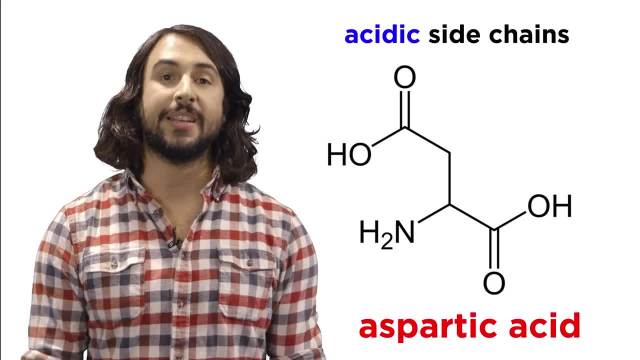 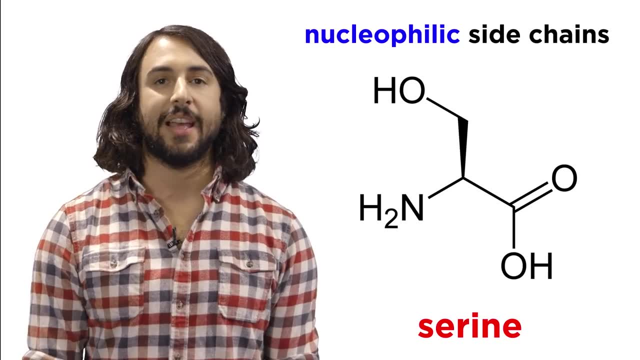 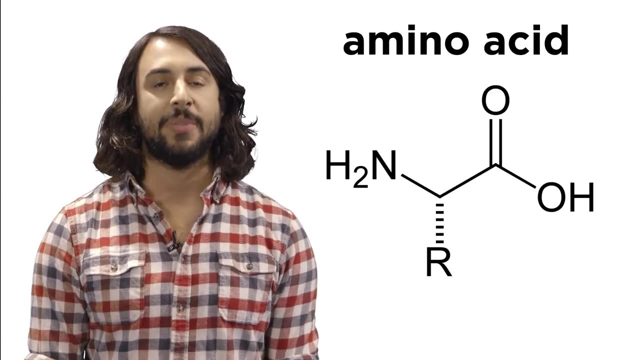 nitrogen atom. Some have R groups that are acidic, like aspartic acid. Some have R groups that can act as nucleophiles, like serine, because of the hydroxyl group. Every amino acid has its own unique structure and reactivity, and it's the variation in 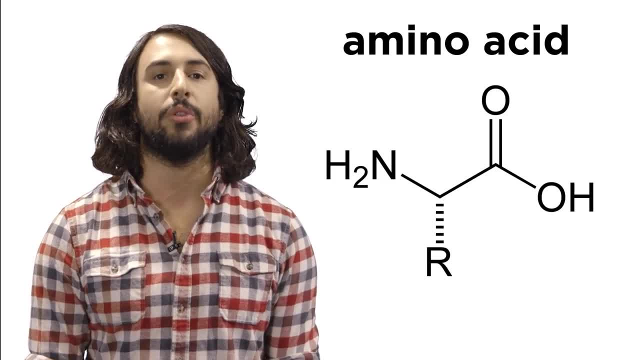 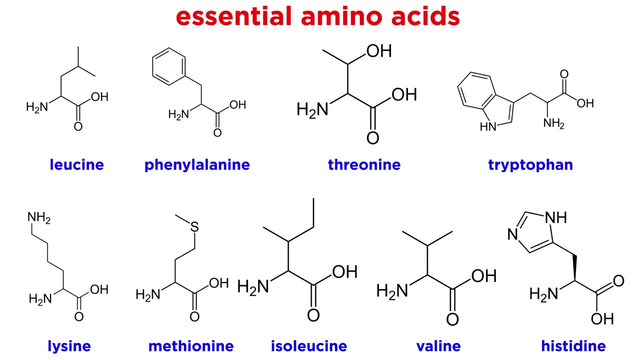 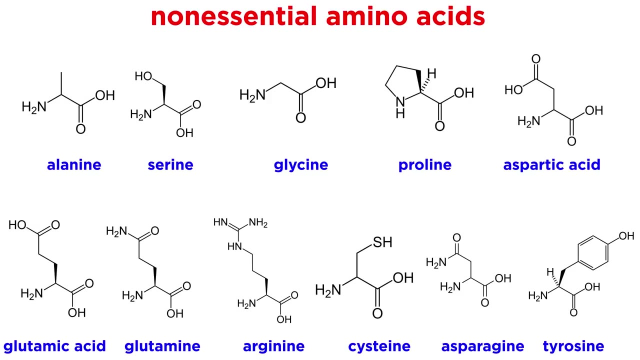 these R groups. that determines the characteristics of the molecule that forms when a bunch of these amino acids join together. Some of these amino acids humans can't make on their own, so we have to eat them in our diet. Others, we are able to make inside our bodies, so those are called non-essential amino acids. 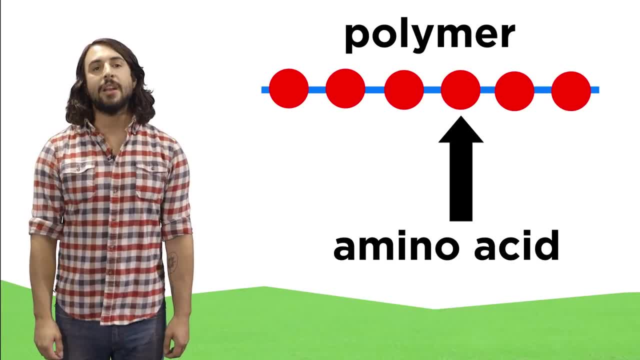 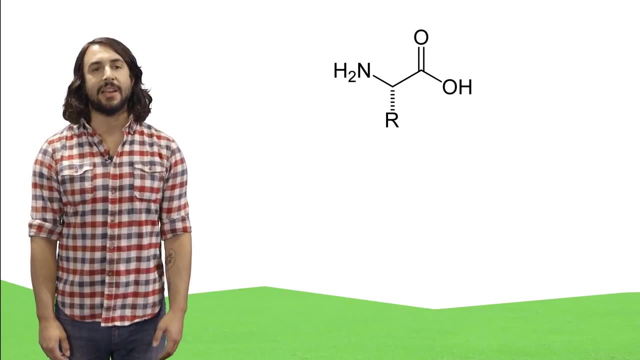 meaning it's not essential that we eat them. So amino acids are monomers, and monomers are the units that join together to form a polymer. How exactly, then, do amino acids polymerize? Before we learn about that, let's first understand that inside the body instead of 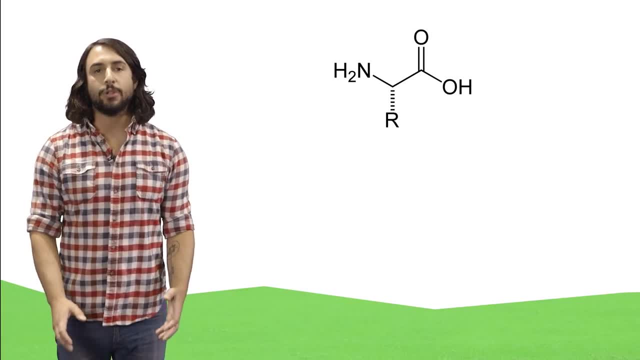 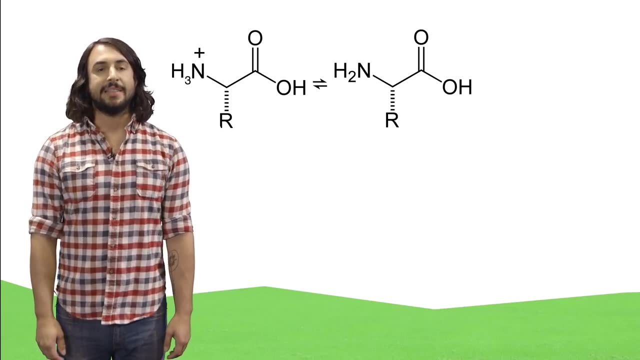 the one structure we've been looking at. there are actually equilibria. There are two structures. There are equilibria between different forms of the amino acid. The amino group can be protonated, since it is slightly basic, and the carboxyl group can. 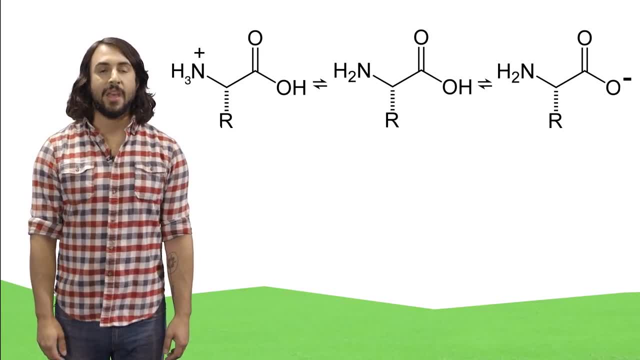 be deprotonated, since it is slightly acidic And there are equilibria between the cationic form, the zwitterionic form and the anionic form. We know what cations and anions are. they're positively charged and negatively charged. 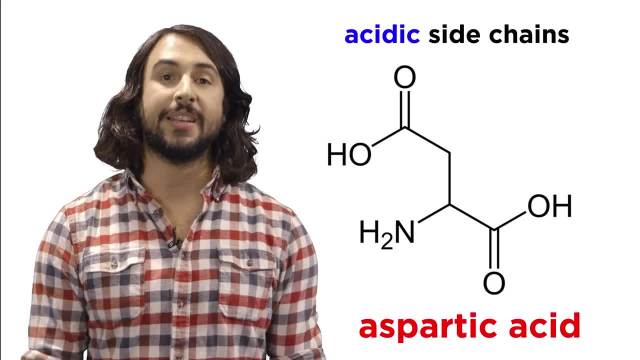 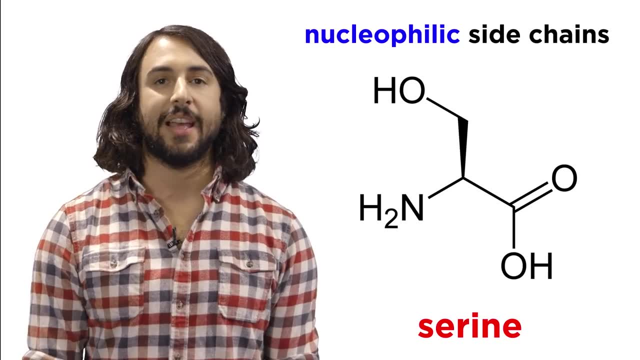 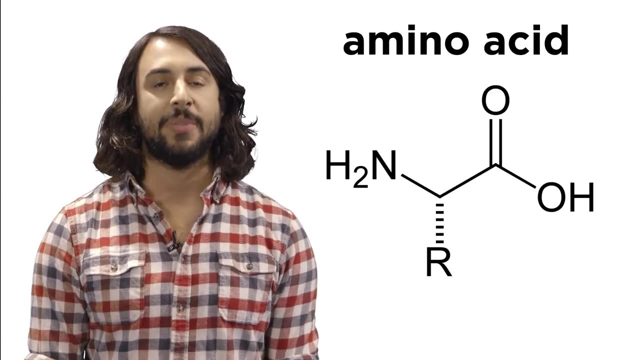 nitrogen atom. Some have R groups that are acidic, like aspartic acid. Some have R groups that can act as nucleophiles, like serine, because of the hydroxyl group. Every amino acid has its own unique structure and reactivity, and it's the variation in 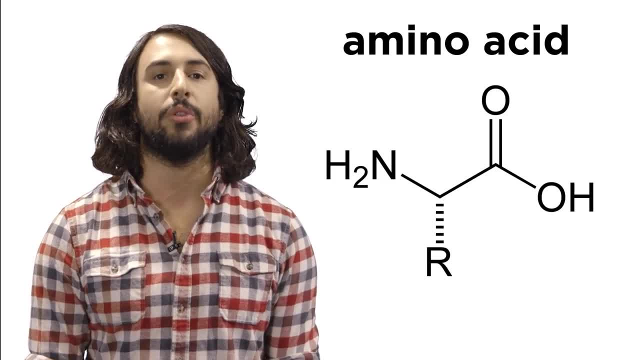 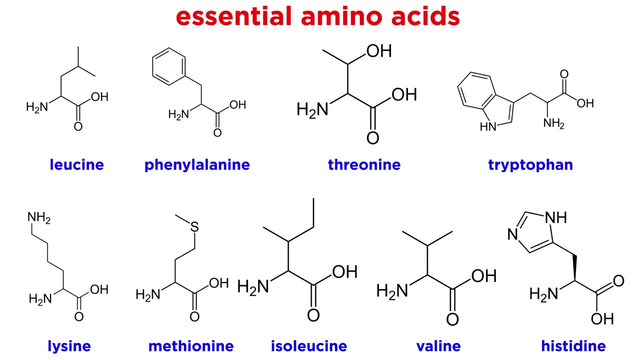 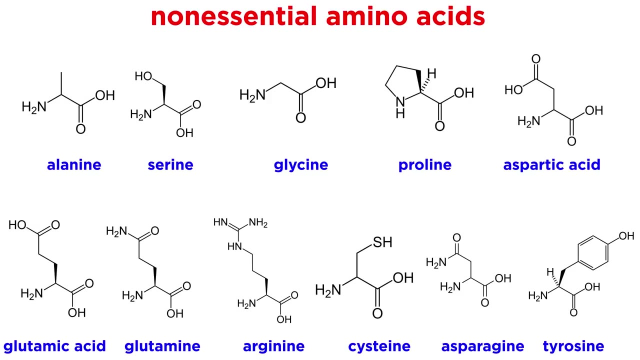 these R groups. that determines the characteristics of the molecule that forms when a bunch of these amino acids join together. Some of these amino acids humans can't make on their own, so we have to eat them in our diet. Others, we are able to make inside our bodies, so those are called non-essential amino acids. 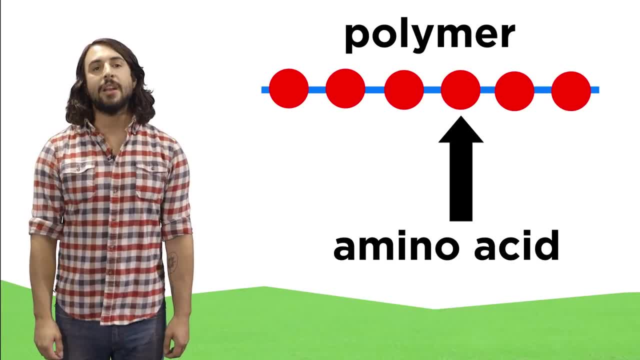 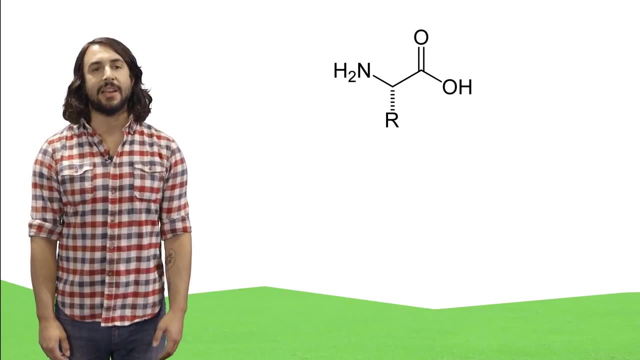 meaning it's not essential that we eat them. So amino acids are monomers, and monomers are the units that join together to form a polymer. How exactly, then, do amino acids polymerize? Before we learn about that, let's first understand that inside the body instead of 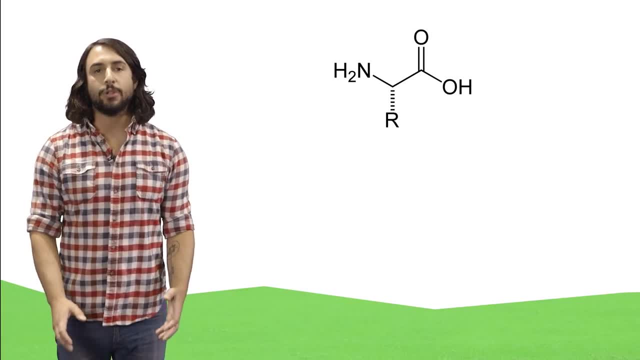 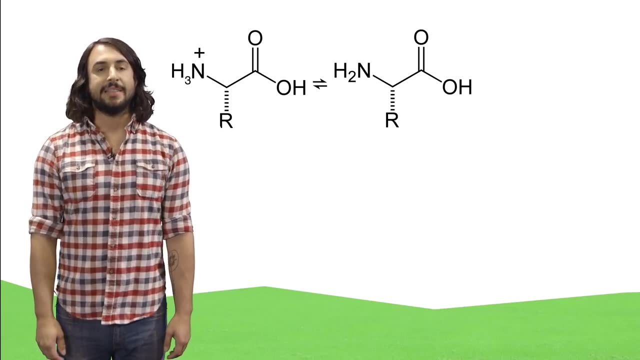 the one structure we've been looking at. there are actually equilibria. There are two structures. There are equilibria between different forms of the amino acid. The amino group can be protonated, since it is slightly basic, and the carboxyl group can. 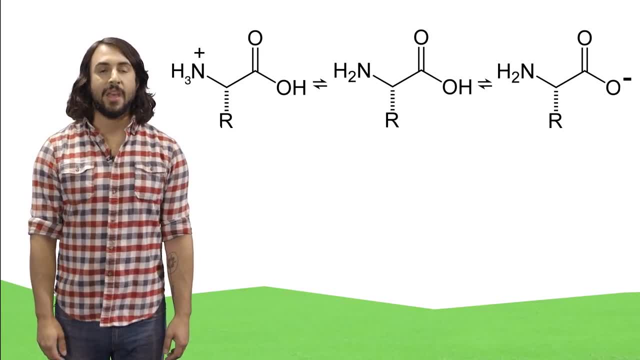 be deprotonated, since it is slightly acidic and there are equilibria between the cationic form, the zwitterionic form and the anionic form. We know what cations and anions are. they're positively charged and negatively charged. 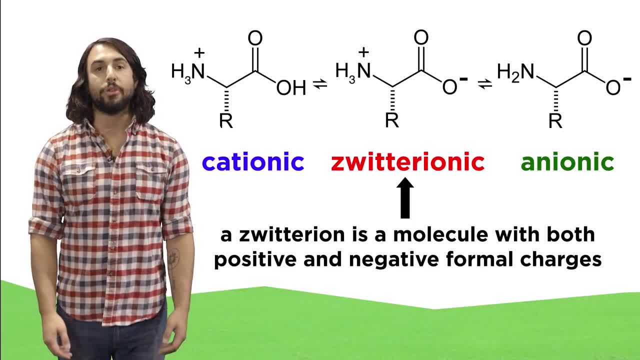 species And a zwitterion is a molecule that has both a positive and a negative charge. The form that an amino acid will take depends on the pH of its environment. A more acidic solution will favor the cationic form, since basic groups will pick up protons. 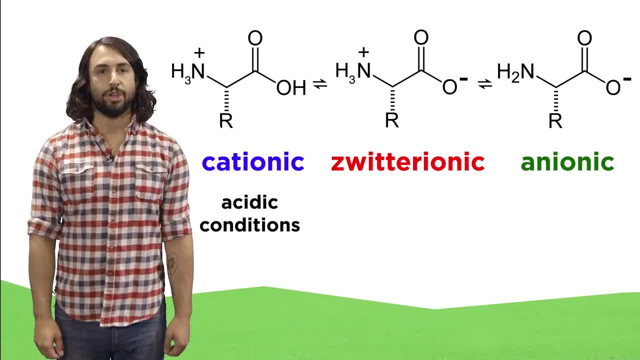 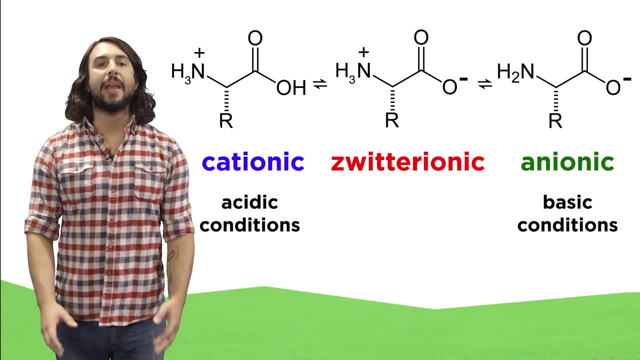 from the hydronium in solution And a more basic solution will favor the anionic form, since acidic groups will readily deprotonate in the presence of hydroxide Inside the body. the pH is regulated very precisely and in most areas of the body it 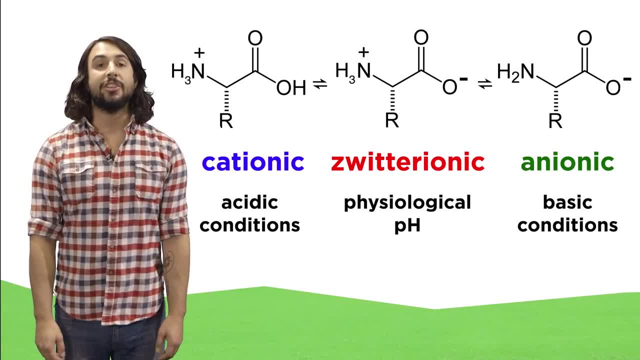 is very 10 times more than in the surface of the body. So the pH of the amino acid is 10 times more in some groups than in other forms, and that's In most areas. it's fairly close to neutral pH. so the zwitterionic form is typically